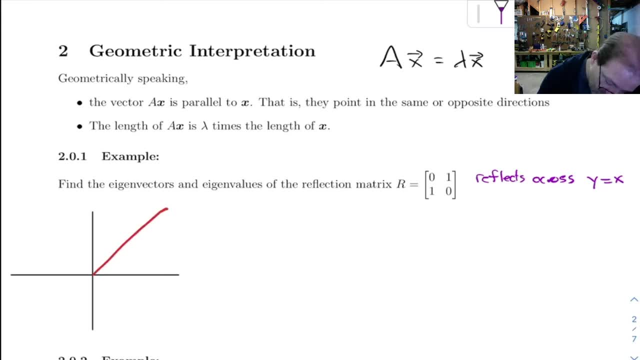 is y equals x. All right, so let's say we have this vector out here, This is going to reflect it across the line up to here. So are there any vectors that this would not sort of change the angle of? And there's one that I think is pretty obvious If you take a point that lies right. 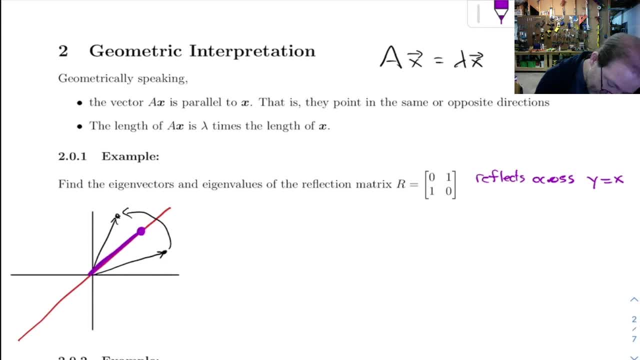 lies on this line. think of it as a point or think of it as a vector. When you multiply that by this matrix, it just swaps x and y. Well, since it's on this curve, here, or on this line, y equals x. it's not going to change. So any vector that lies on this line, the. 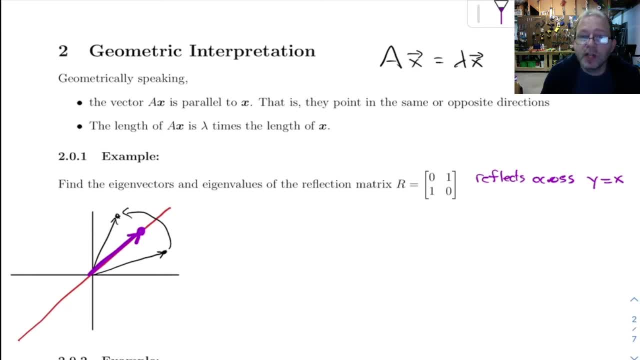 line of reflection is unchanged by this. So vectors on the line y equals x are unchanged. Another way of saying that is they are multiplied by 1.. When multiplied by r, I call this matrix r for reflection. So the eigenvalue is 1.. 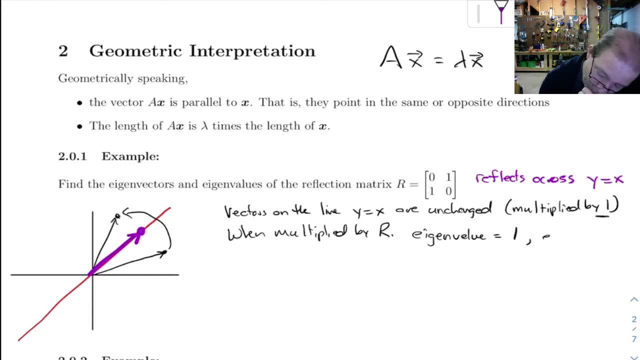 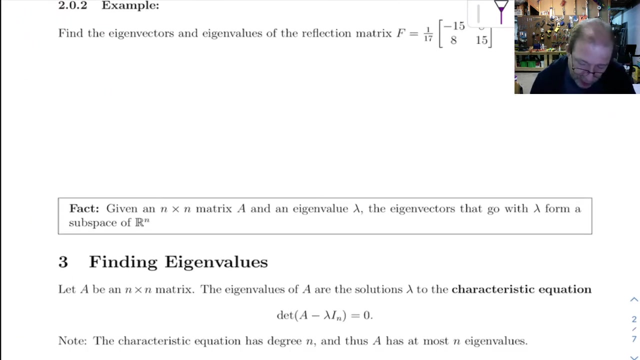 The eigenvectors are all the vectors that lie on that line. Another way we could say: that is the span of. So that's one eigenvalue, eigenvector pair. Now notice the eigenvector. we don't just get one, we get infinitely many of them. That actually sort of foreshadows this down here. 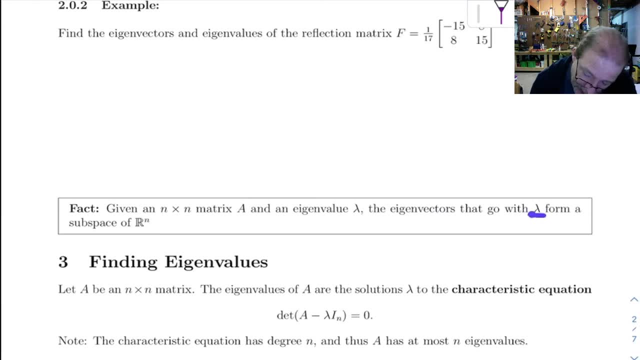 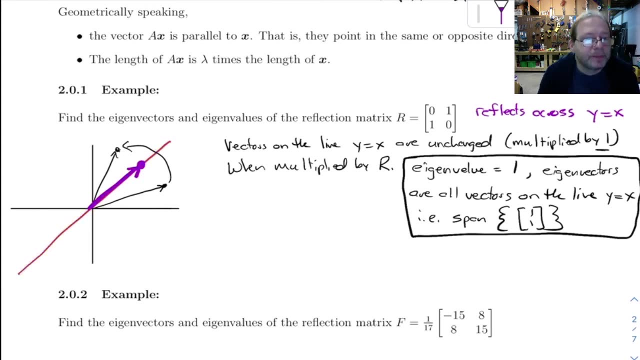 The eigenvectors that go with lambda, a given eigenvalue form a subspace of rn. Sure enough, these form a subspace. It's this line through the origin. Are there any other vectors that this reflection will just either unchange or reverse the direction?